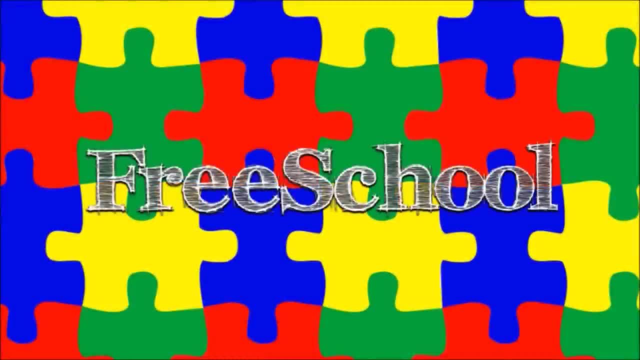 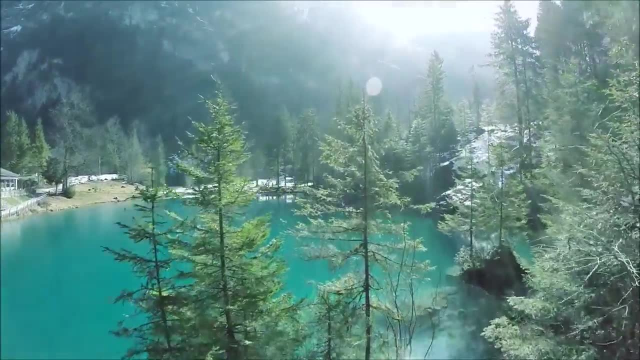 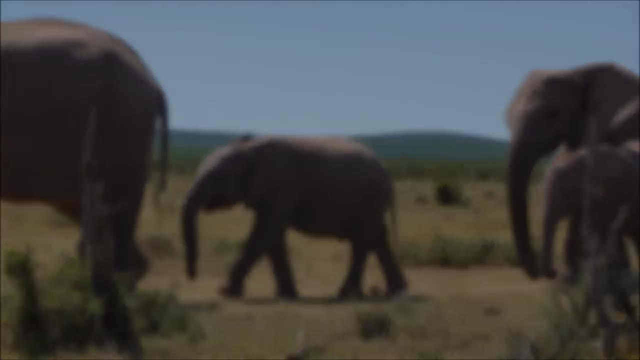 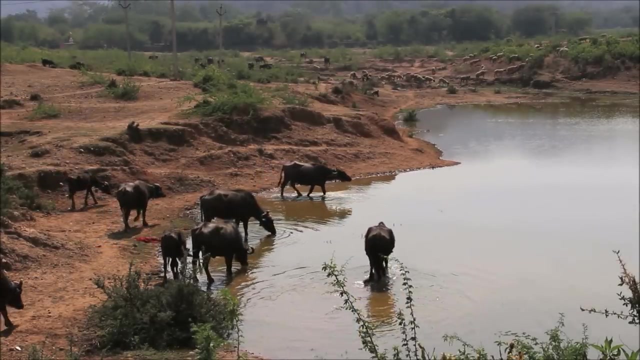 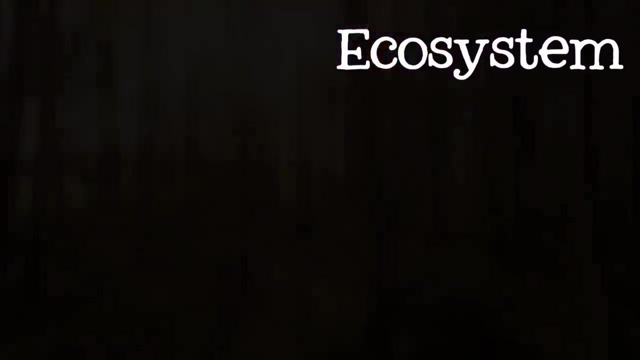 The earth is covered in living things, From very large organisms to the tiniest creatures. all living things on earth have one thing in common – they cannot survive alone. To grow and flourish, living things need the support of an ecosystem. An ecosystem is what we call all the things that interact in a specific area. 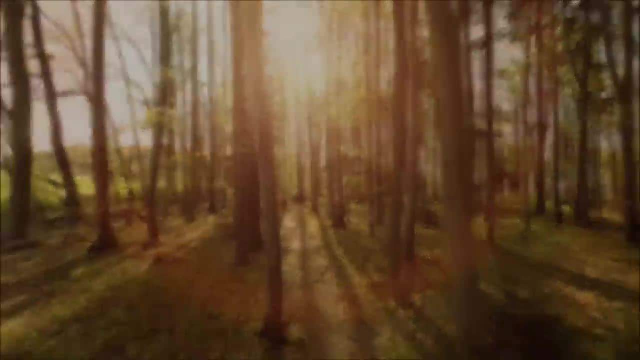 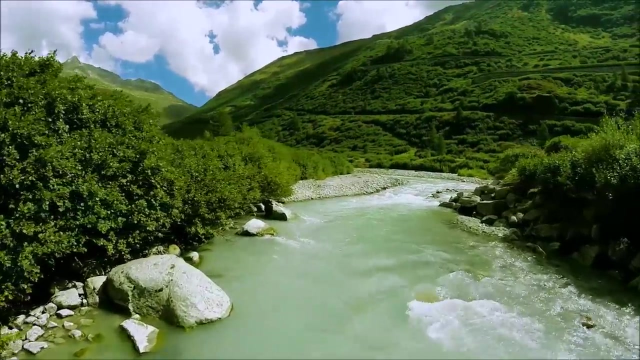 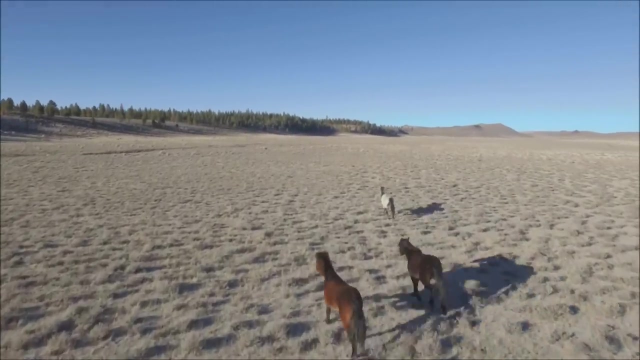 both living and non-living Ecosystems can be hard to define. They are interconnected in many ways and it is not always easy to see where one ecosystem ends and another begins. Different ecosystems may look very similar or very different from one another, but all ecosystems. 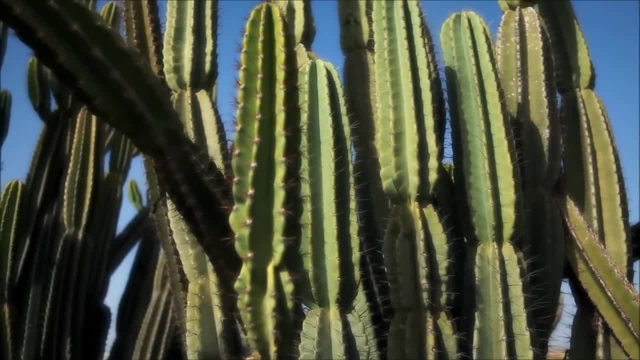 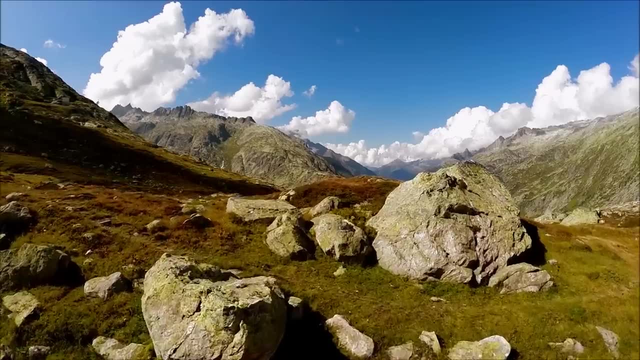 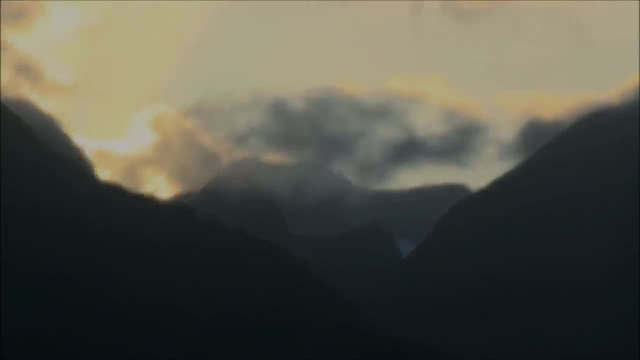 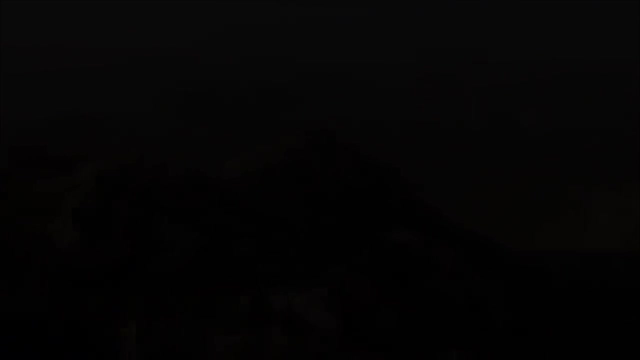 are made of the same basic parts. Ecosystems have both living and non-living parts. The non-living parts of an ecosystem include things like sunlight and temperature, air and wind, the types and amount of water available, and rocks and soil. 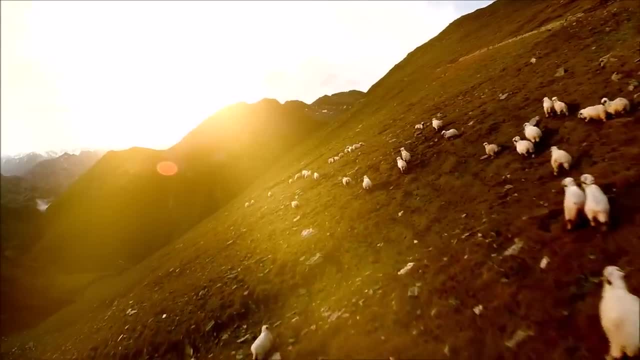 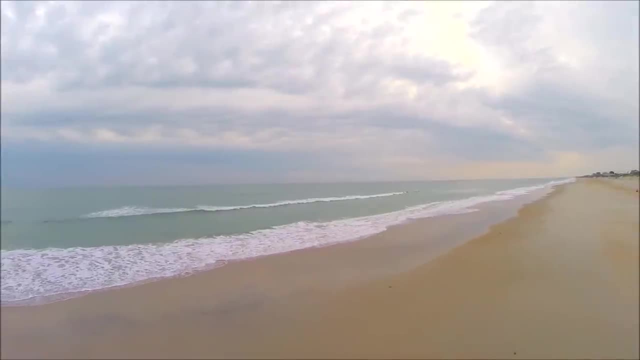 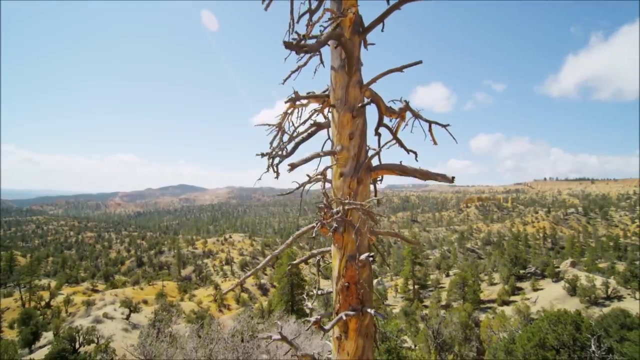 The living parts of an ecosystem are the plants and animals in it. The non-living parts of an ecosystem combine to create the conditions that will determine what kinds of living things will be able to survive there. You won't find a coral reef in the desert or cactus in the ocean, because the conditions 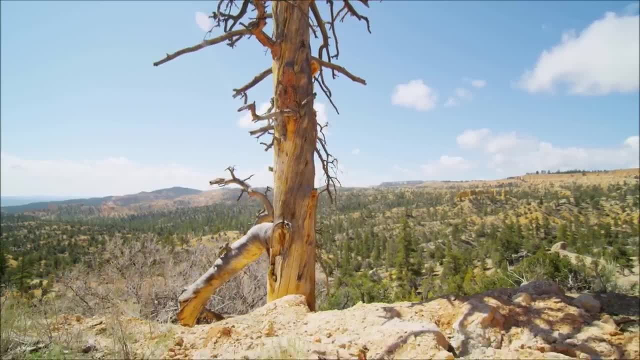 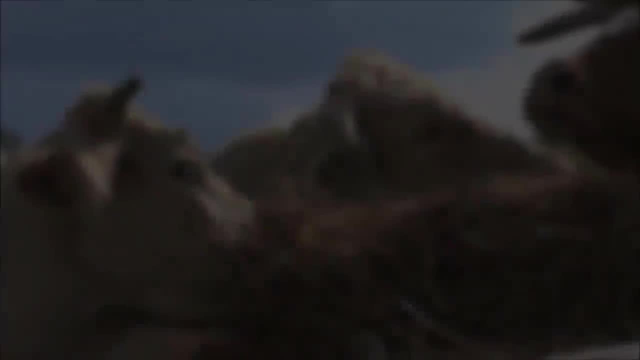 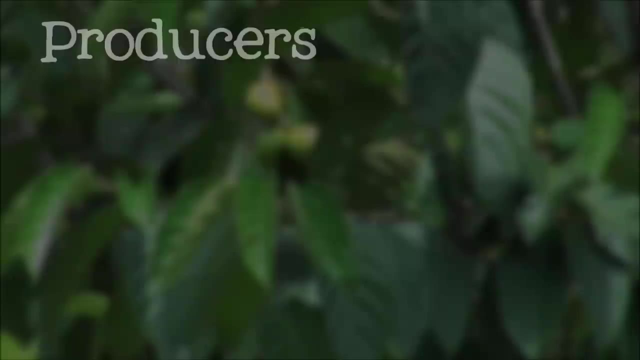 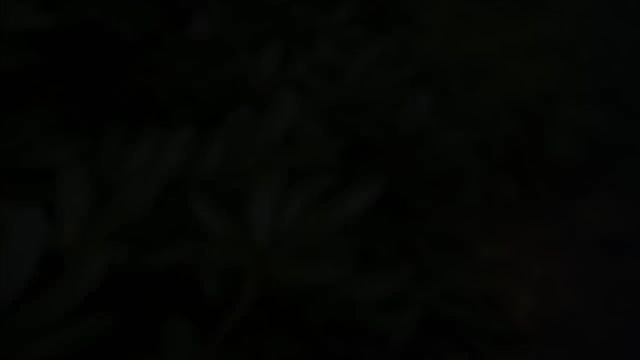 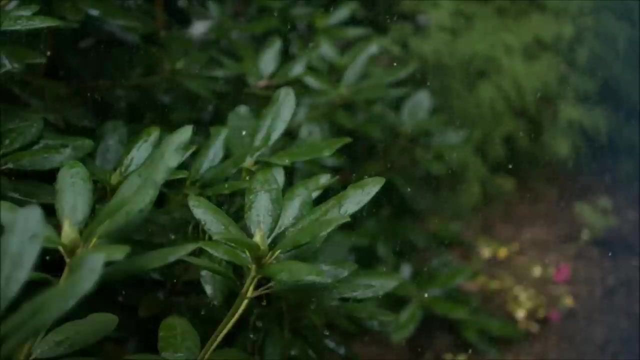 are wrong for them to live and grow. There are three main types of living things in an ecosystem – producers, consumers and decomposers. Producers produce or make their own food. Usually they make their food from sunlight through photosynthesis. Plants are the most obvious example of producers Without producers. 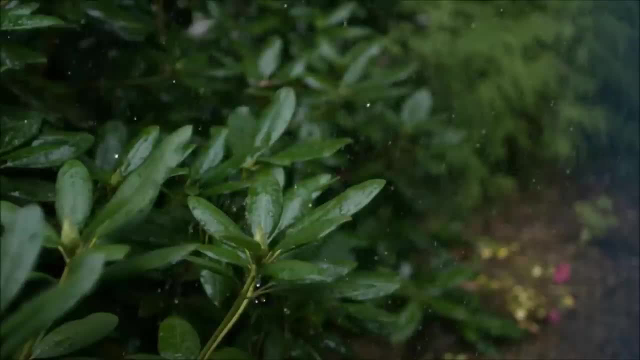 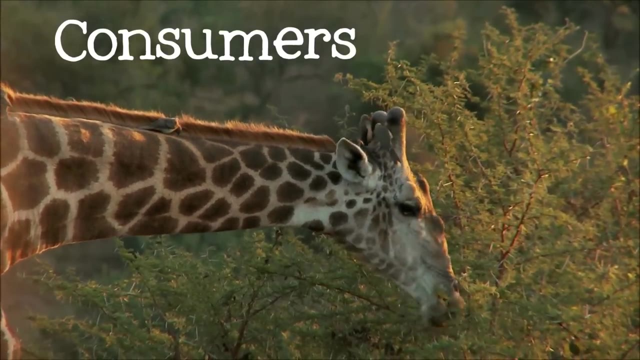 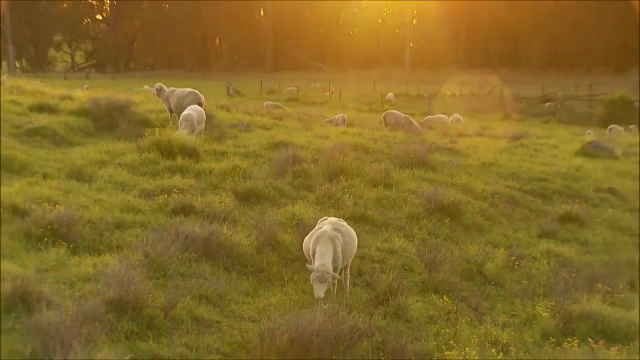 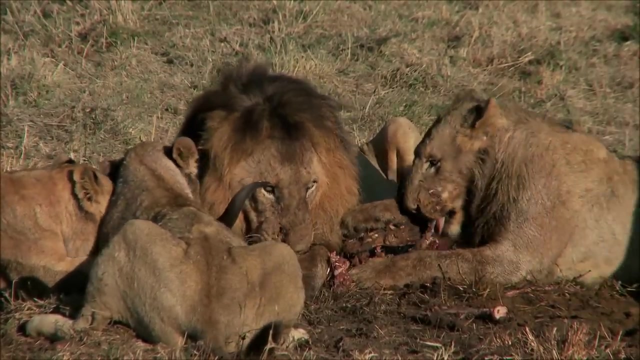 no animal would be able to survive. That's because all animals are consumers and need to consume or eat their food. Some animals, called herbivores, get their energy from eating plants. Other animals, called carnivores, get their energy from eating other animals. 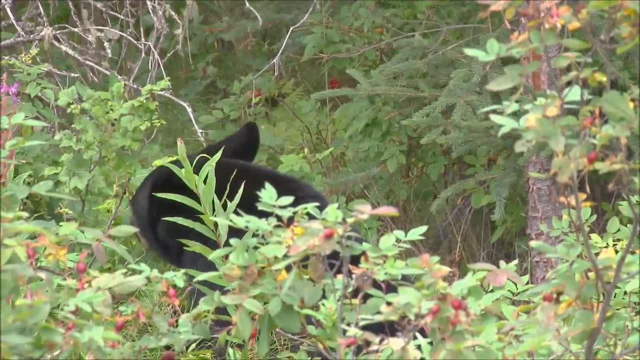 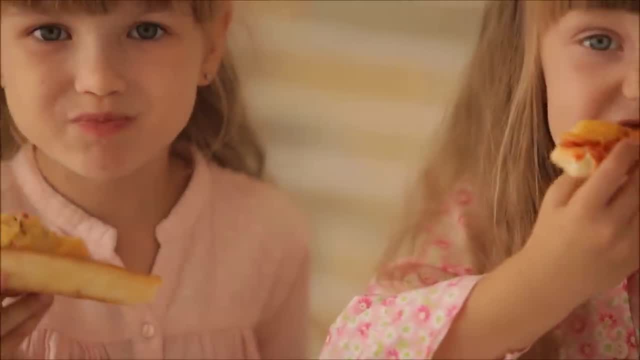 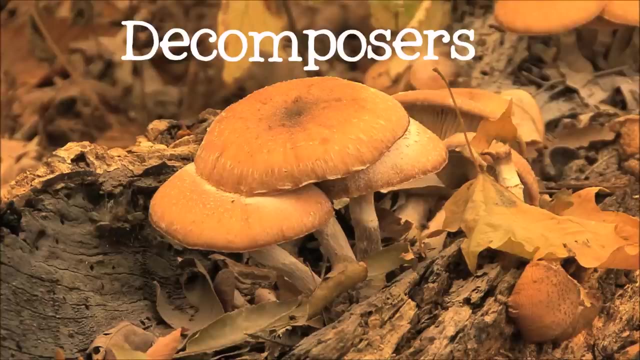 There is a third group of animals called omnivores. Omnivores get their energy by eating both plants and meat. Humans are an example of omnivores. Finally, plants. Finally, there are the decomposers. Decomposers are generally bacteria and fungi They consume. 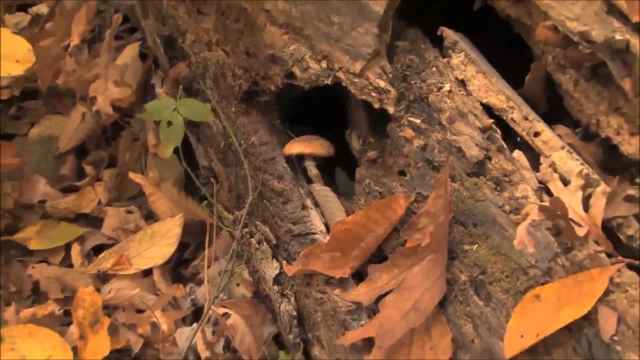 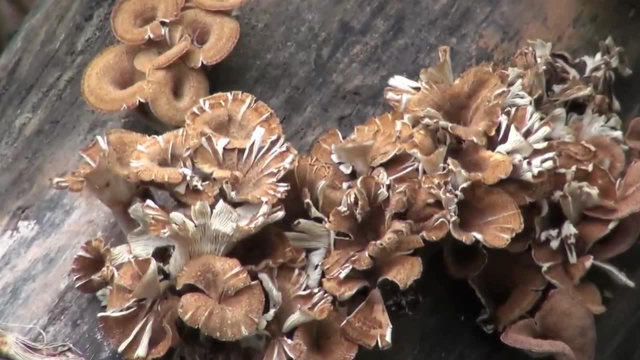 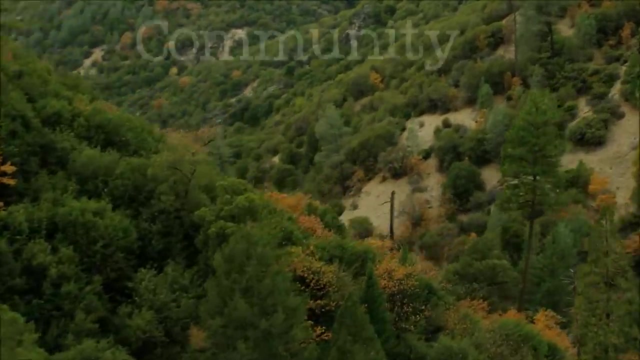 dead plants and animals and break them down into nutrients that are released into the soil. These nutrients are used by producers like plants to help them grow, and the cycle begins all over again. The living things inside an ecosystem form a community. Within the community are many different species. Some plants have a unique, unique, unique. 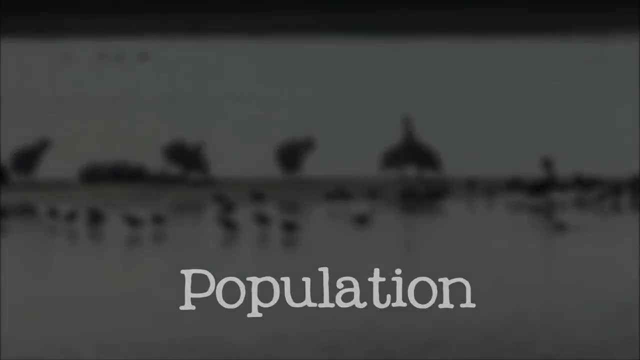 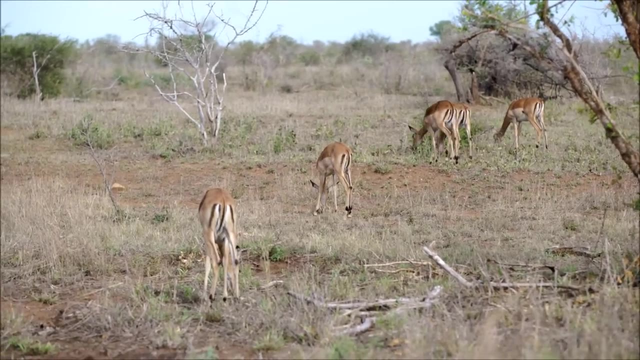 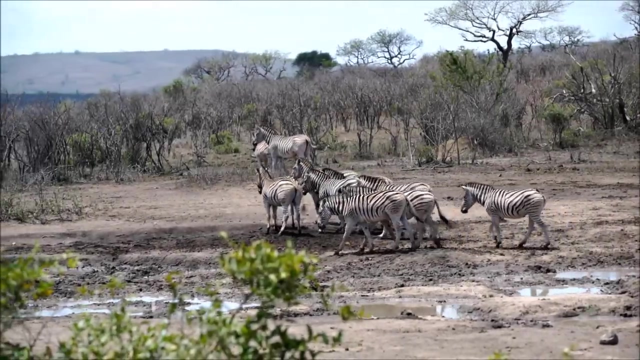 population. A population is made of all the members of one specific species. For instance, all of the plants and animals on the savanna make up the savanna community. Within the savanna, all of the zebras make up the zebra population. all of the acacia. 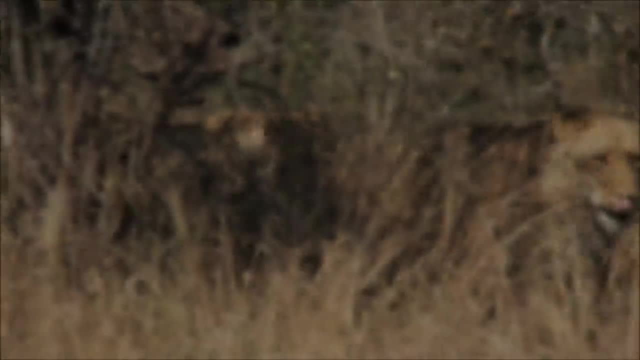 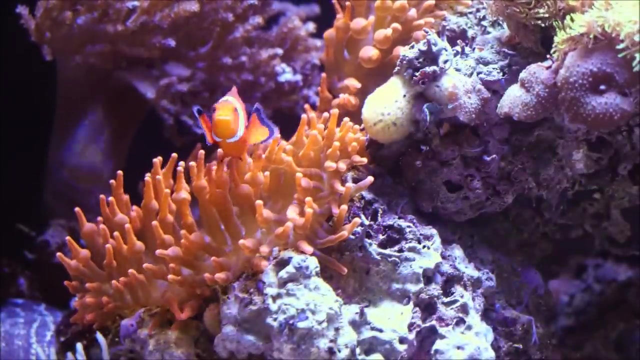 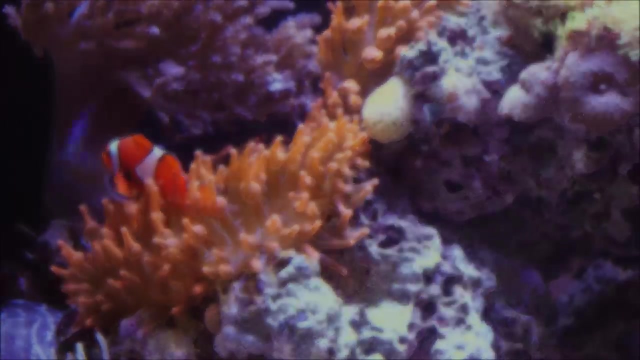 trees make up the acacia tree population and all of the lions make up the lion population. All the parts of an ecosystem must work together to reach a balance that allows each of the members of the system to thrive. For example, in a balanced ecosystem, predators keep the population of rabbits from growing. 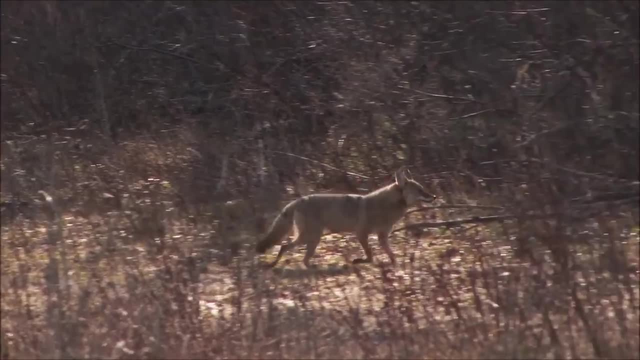 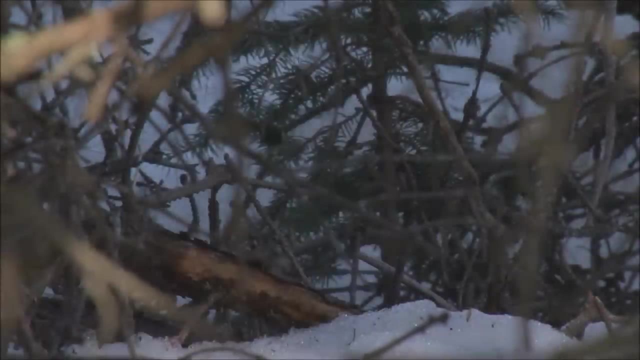 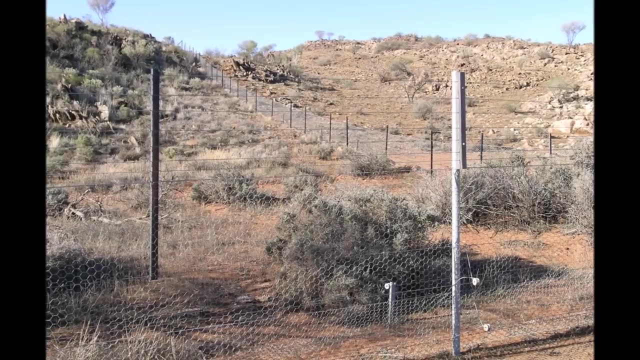 too large, because when there are too many rabbits, they eat too many plants. If rabbits ate too many plants, the plants would not be able to grow back fast enough and other animals that need the plants would not have enough to eat. Without enough plants, the animals that depend on them for food would start to die, and